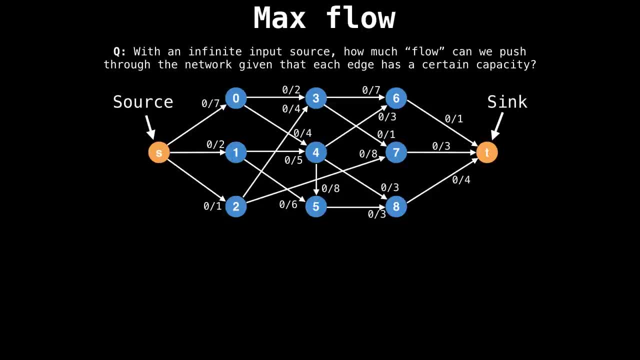 called a flow graph. This is a graph where edges have a certain maximum capacity which cannot be exceeded. Edges also have a flow value, which is how many units of flow are passing through that edge. Initially, the flow is zero for all edges, everywhere, until 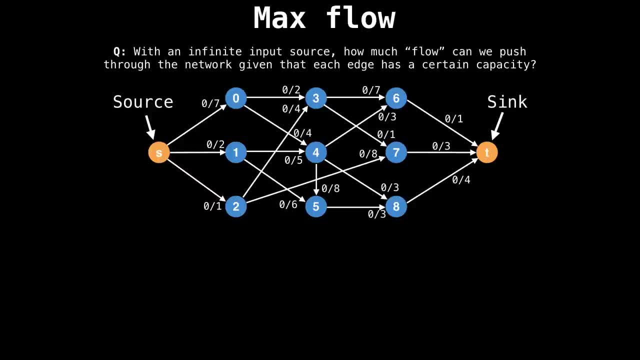 we run a max flow algorithm on it. There are also two special types of nodes in the flow graph: the source node and the single node, Usually denoted as s and t respectively. The maximum flow problem asks, with an infinite input source, how much flow can we push through the network without exceeding the capacity? 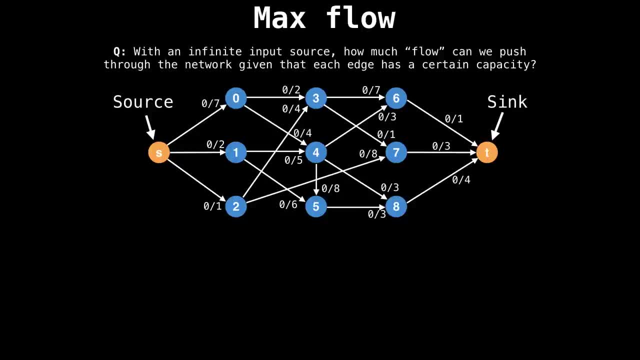 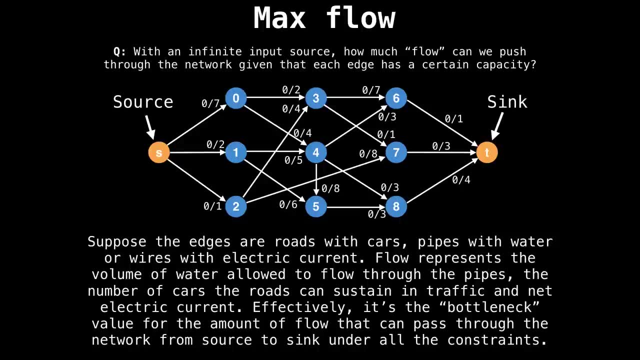 of any edge, and it's not all obvious how one should figure that out. Maximum flow can be used in numerous situations where edges and nodes can represent any number of things. For instance, suppose the edges are roads, cars or pipes with water, wires, with electric current and 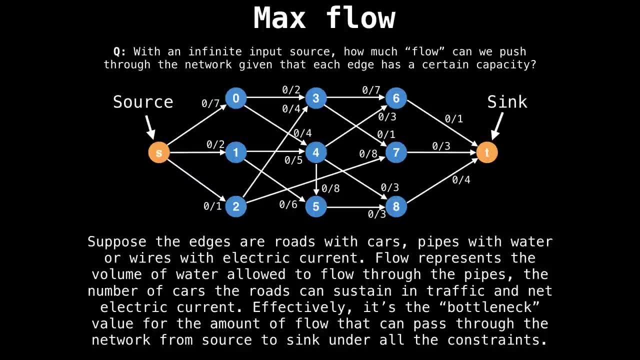 so on. Each of those has a certain capacity value we can associate with the maximum flow, on the other hand, would represent the volume of water that can flow through the pipe. So the number of cars the roads can sustain in traffic, or the net electric current that your 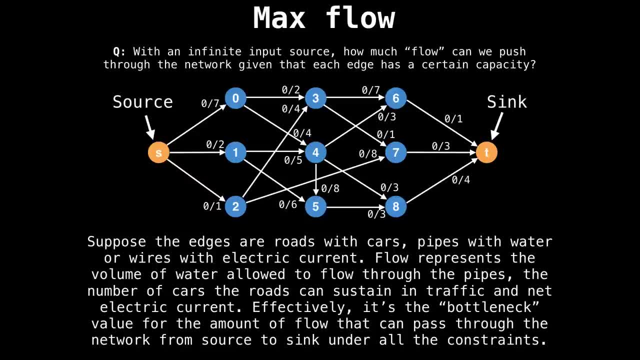 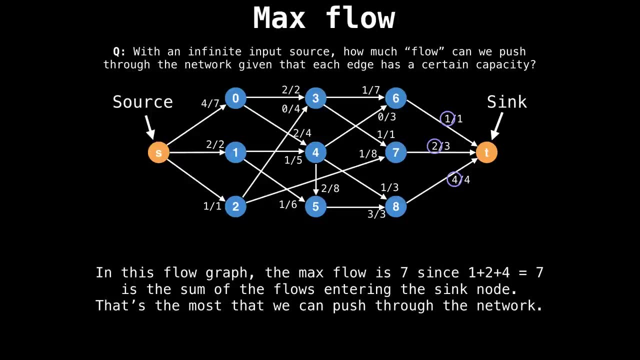 system can sustain Effectively. the maximum flow is a bottleneck value for the maximum flow of traffic your network can handle, And that is going from the source to the sink. under all those constraints, The maximum flow for this particular network is seven, And you can tell because, after running the maximum flow algorithm, the sum of the flows 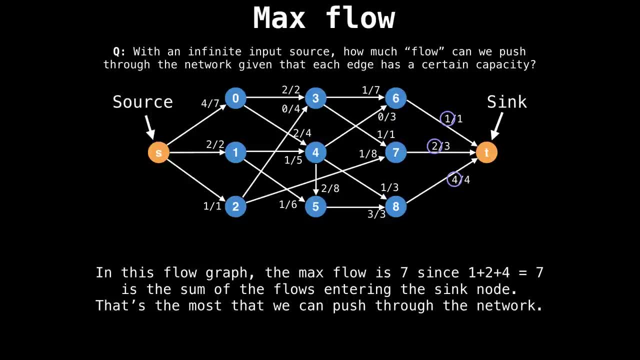 attached to the sink node is seven Running. a maximum flow algorithm is used to determine how much flow each edge should receive to achieve the overall maximum flow. Note that there might be multiple ways of achieving the maximum flow, by giving each edge different flow values, but overall solutions will have the same maximum flow value. Let's 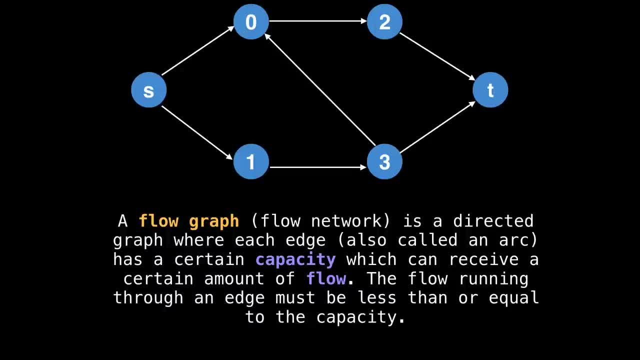 dig deeper into how to find the maximum flow. To begin with, you will need a flow graph which consists of directed edges, which are also called arcs. Each directed edge has a certain capacity which can receive a certain amount of flow. At all times, the flow running through an edge must be less than or equal to the capacity. 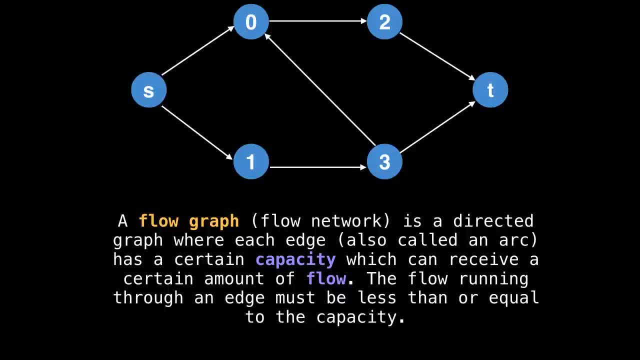 This intuitively makes sense, Because if we allow more flow than what the capacity permits, it means something has to go wrong. When an edge becomes overcapacitated in some manner, it means that we've pushed the system past its limit. In the context of edges representing 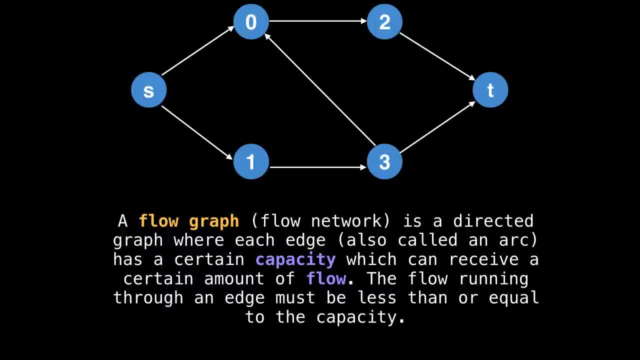 pipes with water, it means your pipe broke or it leaked. If your edge is a wire with electric current, It means your wire literally fried or melted, exploded or something bad happened to it because there was too much electric current. This is not good, So this is why we don't allow. 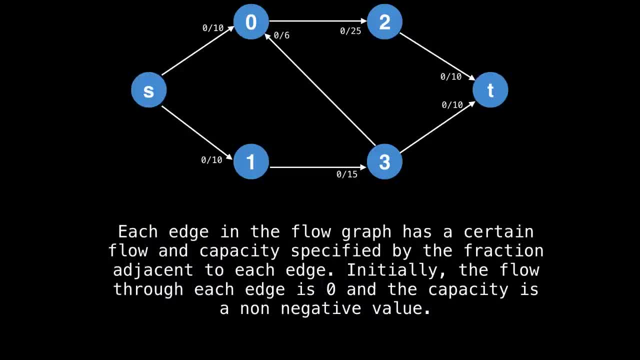 more flow than capacity. Each edge in the flow graph has a certain flow and capacity specified by the two values separated by a slash adjacent to each edge. Originally, the flow through each edge is zero and the capacity is a non negative value to find the maximum. 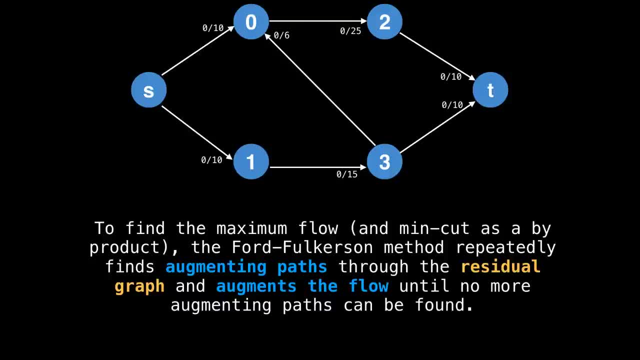 flow. This is also the min cut. as a byproduct, The Ford Fulkerson method repeatedly finds augmenting paths through the residual graph and augments the flow until no more augmenting paths can be found. So you're probably asking yourself at this moment: what is an augmenting path? 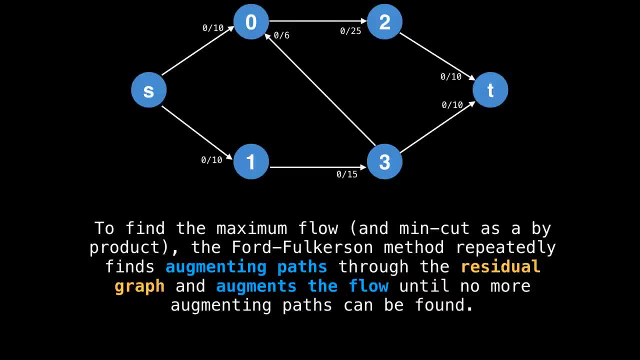 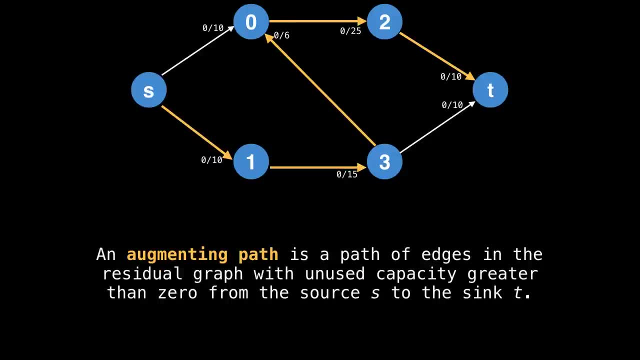 What the heck is a residual graph? And what do you mean by augment the flow? All right, let me explain. We'll do them one by one. An augmenting path is a path of edges, that is, in the residual graph with capacity greater than zero, from the source s to the sink t. 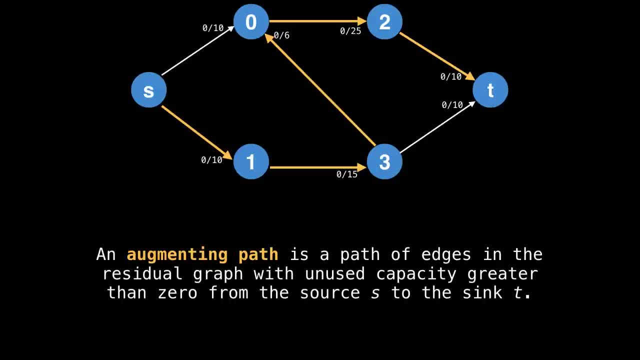 In orange. here I have highlighted a possible augmenting path. The key thing to remember about an augmenting path is that it can only flow through edges which aren't fully saturated yet. In fact, you know you've achieved the maximum flow when there are no more augmenting. 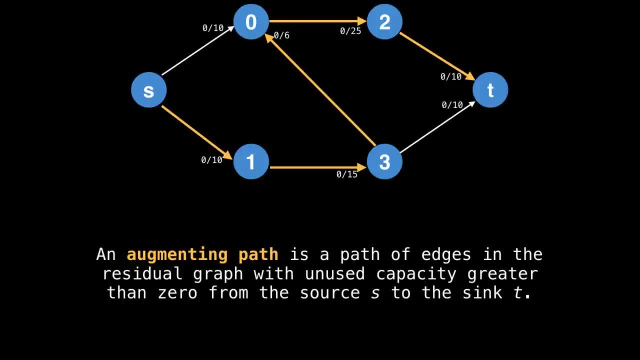 paths left to be found. How to actually find an augmenting path is a deep dive into the detail left unspecified by the Ford Fulkerson method for flexibility. For now, let's assume that we're using a depth for search. Something else to know is that every augmenting path 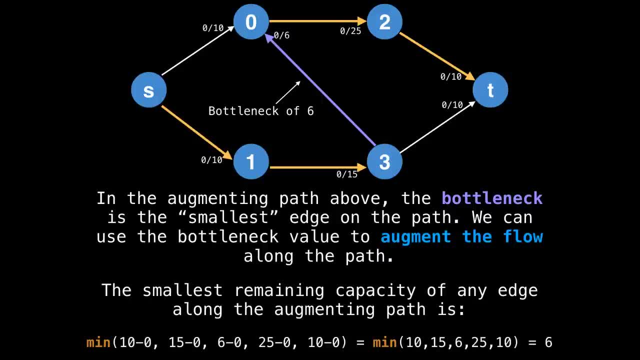 will have what I call a bottleneck value, which is the smallest edge along the path. you can find the value of the bottleneck by taking the difference between the capacity and the current flow of an edge For this augmenting path. the bottleneck value is: 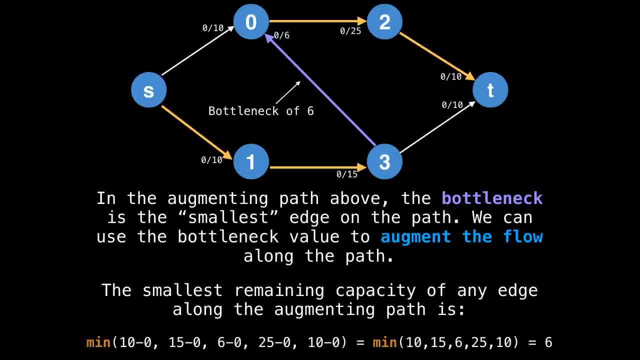 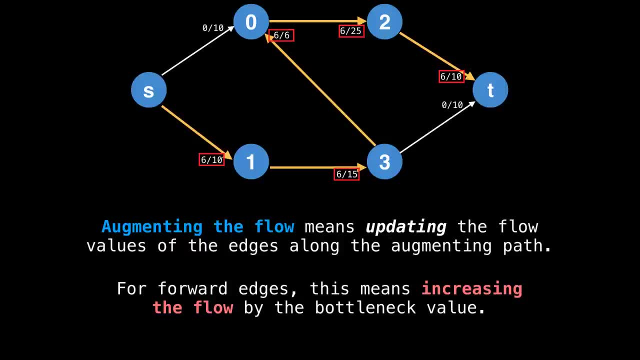 six. we can use the bottleneck value To argument the flow along the path. augmenting the flow simply means to update the flow values of the edges along the augmenting path. Here you can see that I've increased the flow of each edge along the augmenting path by exactly six units. However, we're not done augmenting. 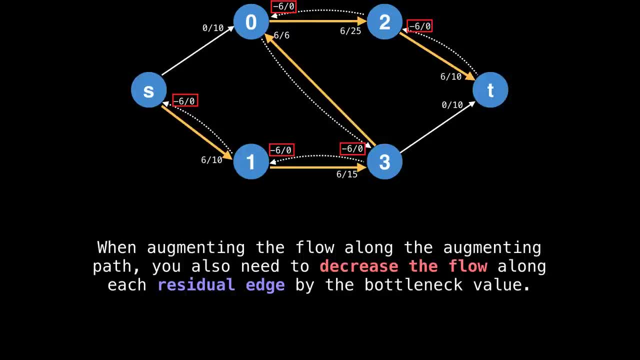 the flow. we not only need to increase the flow along the forward edges, but also decrease the flow along the backwards edges, which are called the residual edges. Okay, the residual edges are the dotted edges going backwards, in the reverse order of the augmenting. 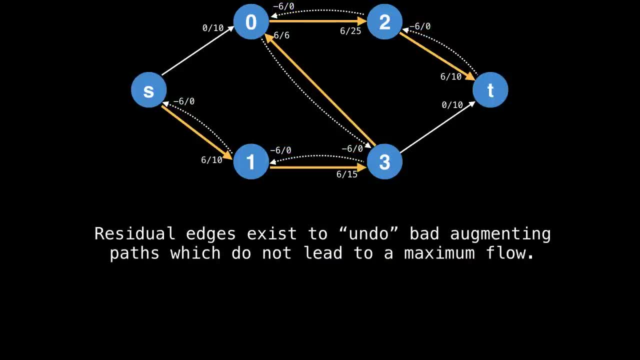 path. The logic behind having residual edges is to undo bad choices of augmenting paths which do not lead to a maximum flow. Effectively, we don't know which are the best, or even correct augmenting paths to take, So this mechanism enables us to freely find any augmenting paths. 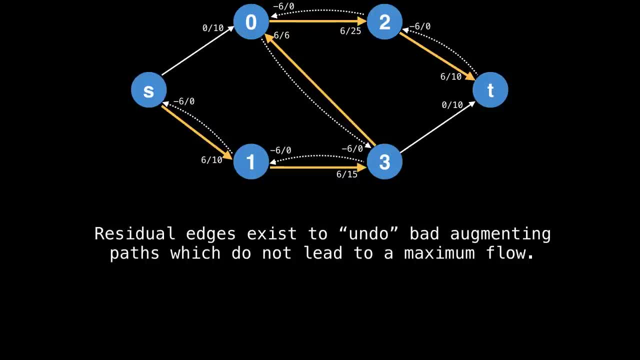 without having to worry about whether or not we'll be able to find any augmenting paths, without having to worry about whether or not we'll be able to achieve the maximum flow. it should be mentioned that residual edges become valid edges to take when finding an. 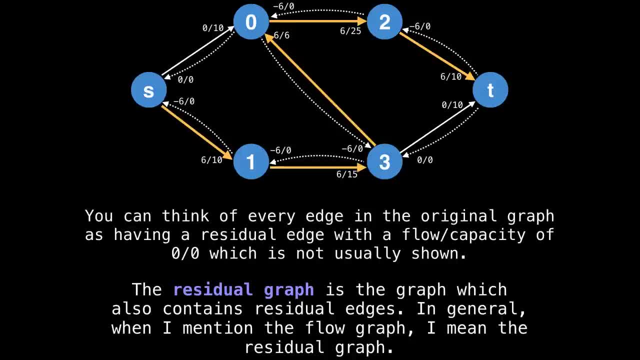 augmenting path in later iterations. So if we take a step back, you can think of every edge in the original graph as having a residual edge with a flow and capacity of zero which is not usually shown. Now that we know what residual edges are, the term residual graph. 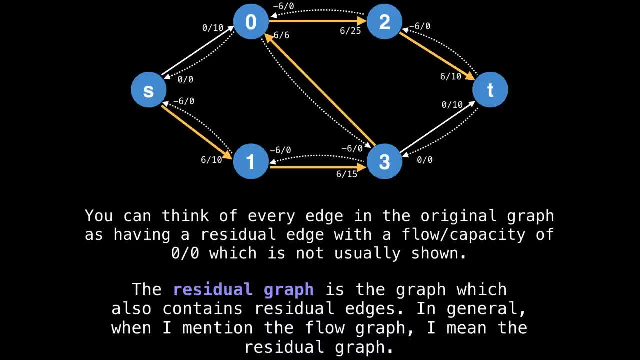 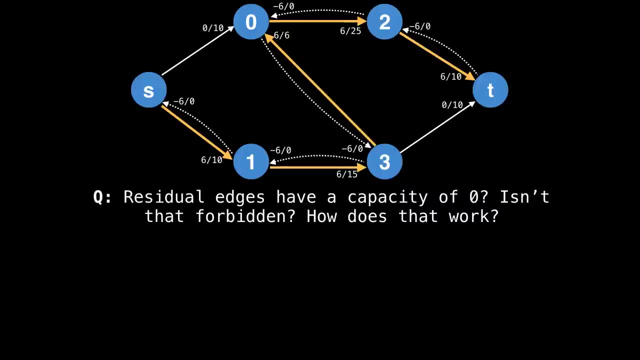 simply means the graph which also contains residual edges, not just the original edges given in the flow graph. So, generally speaking, when I mentioned the flow graph, I usually mean the residual graph. So here's a good question you might have at this point. the 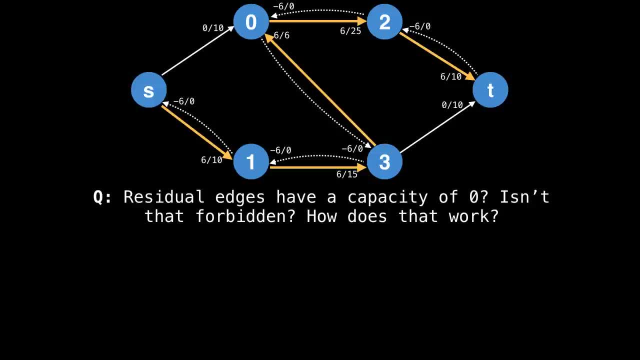 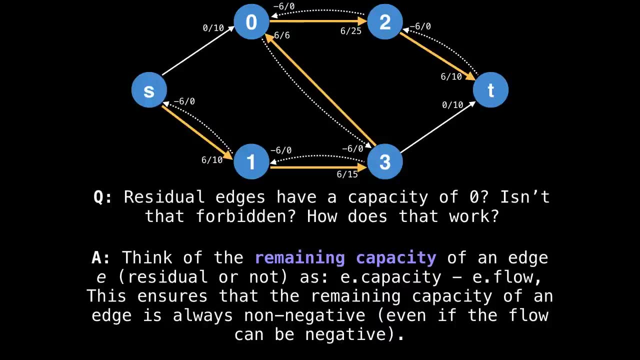 residual edges shown have a capacity of zero, aren't those forbidden? How does that work? So here's the thing. With this method of augmenting the flow, you have to think of the remaining capacity of an edge, E residual or not, as the difference between the capacity. 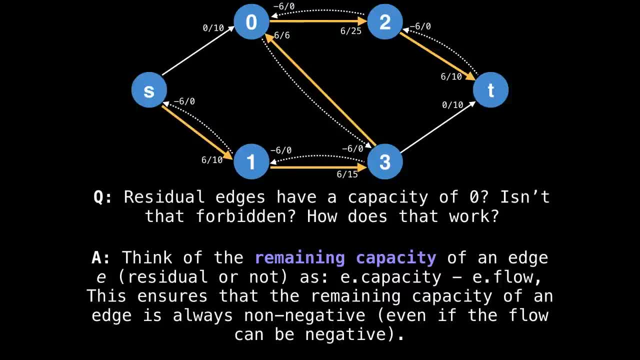 and the flow of that edge- That is, the difference between the capacity and the flow- is the true remaining capacity for that edge. This ensures that the remaining capacity of an edge is always non negative, even if the flow can be negative, For example in the residual. 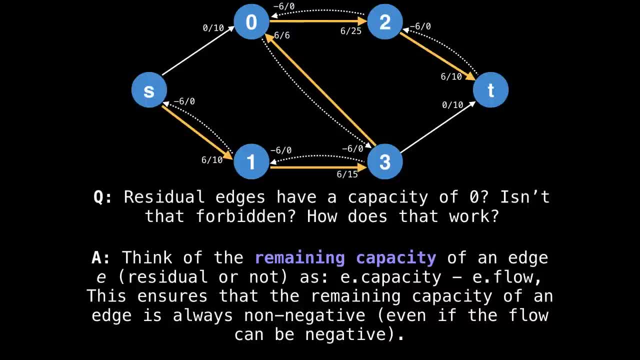 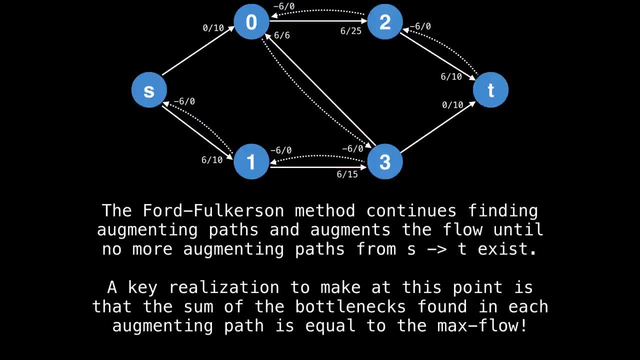 edges we have right now. zero minus minus six is six, So we know that all our residual edges actually have a remaining capacity of six. So the algorithm proceeds and the Ford Fulkerson method continues to repeatedly find augmenting path after augmenting path and to augment the flow until no more augmenting paths from s to t can be found. 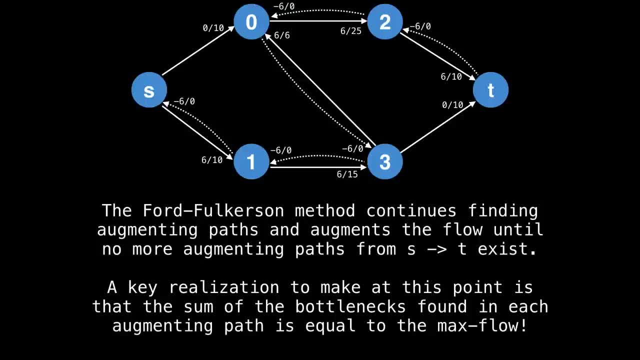 The key realization to make at this point is that the sum of the bottleneck values that we acquire with each augmenting paths will result in the maximum flow, And that's what the whole premise of this algorithm. it doesn't matter so much how you find augmenting paths. 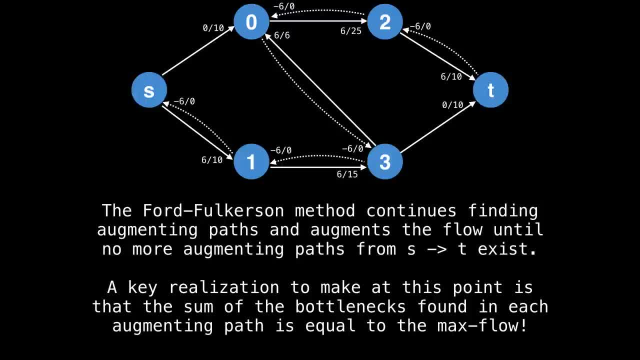 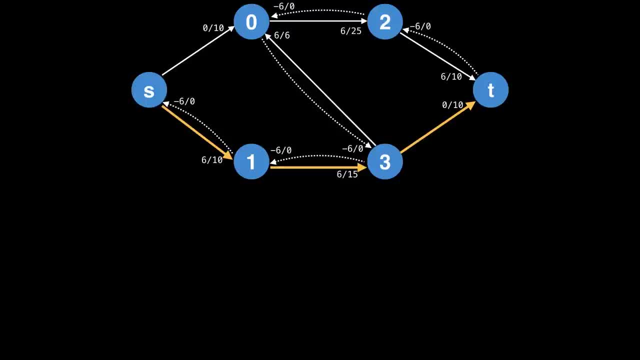 but so long as you keep summing the bottleneck values which they produce, you'll find the maximum flow. So let's keep finding augmenting paths. Remember that we can only select edges whose remaining capacity is greater than zero to be part of the augmenting path. So the 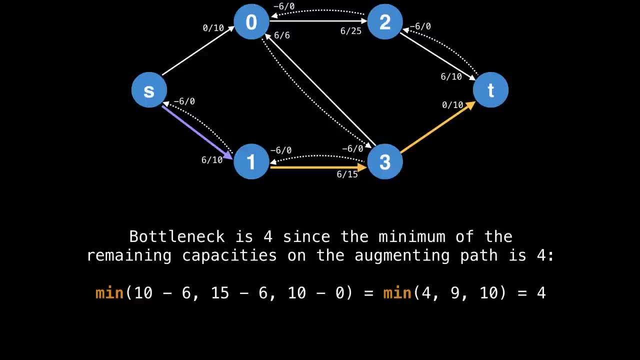 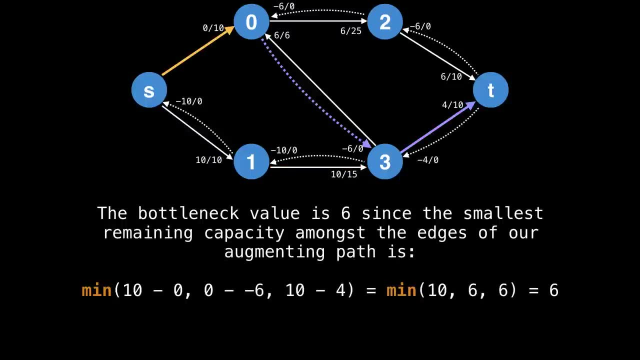 bottleneck for this augmenting path is four, Since we have a minimum of all the remaining capacities along this augmenting path. here's another augmenting path: from the source to the sink. you'll notice that we're actually using one of the residual edges we created earlier in this path. you'll also notice that there are 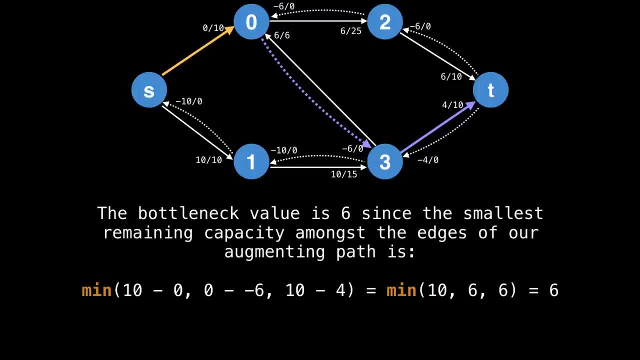 two purple edges in this slide. This is just a coincidence, since both of those edges have the same bottleneck value of six. then we augment the flow as we do. I'll let the animation play for a moment. So let's go ahead and create a new path. So I'm going to create a new path. 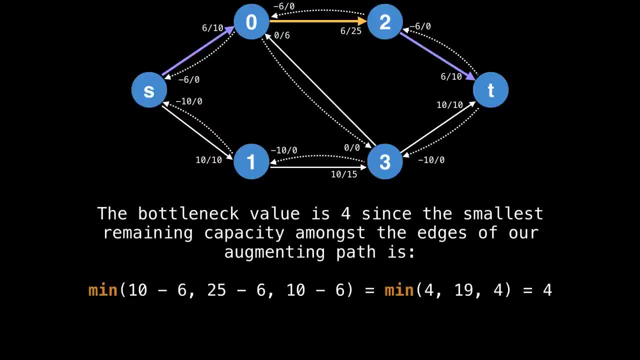 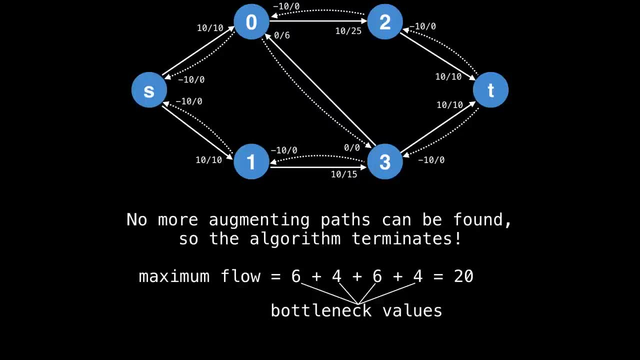 For this next one. And at the end we can see that if we sum all our bottleneck values- six, four, six and four- we're able to achieve the maximum flow, which is 20.. In terms of the time, complexity: 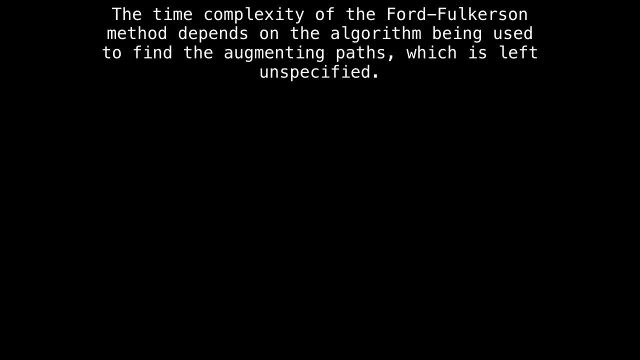 the Ford Fulkerson method derives its complexity from how we actually find those augmenting paths which, as we know, is a very complex method. So let's go ahead and create a new path. F is left as an unspecified detail. if you assume that finding augmenting paths are found, 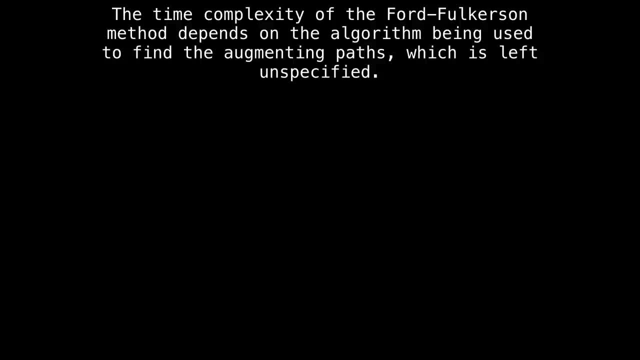 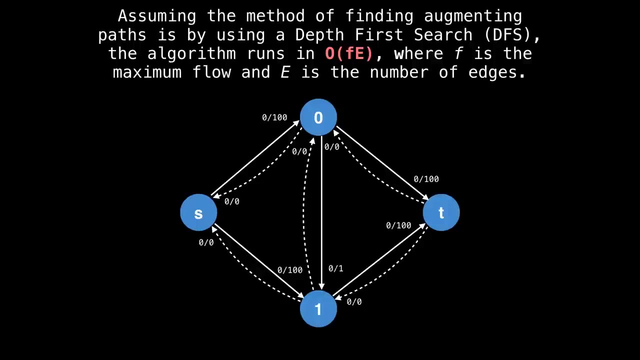 by doing a depth first search. then the algorithm runs in a time complexity of a big O, of, F being the maximum flow times, e the number of edges in the graph. here's a graph. we can derive the time complexity. suppose that the side edges have very high capacity values. 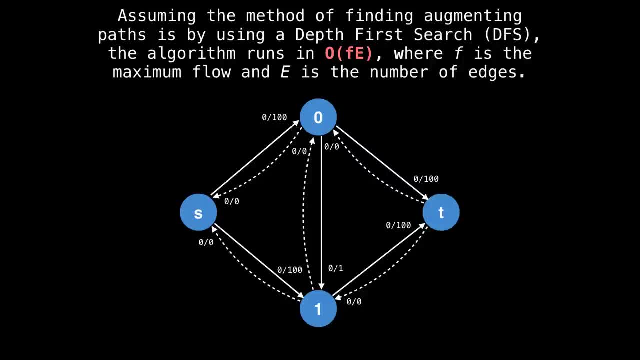 of 100. And the middle edge has a capacity of one, you can clearly tell that the maximum flow should be 200. Because you can run two augmenting paths with flow values of 100 on the top and the bottom of the graph, from the source to the sink. However, recall that a depth first search traversal. 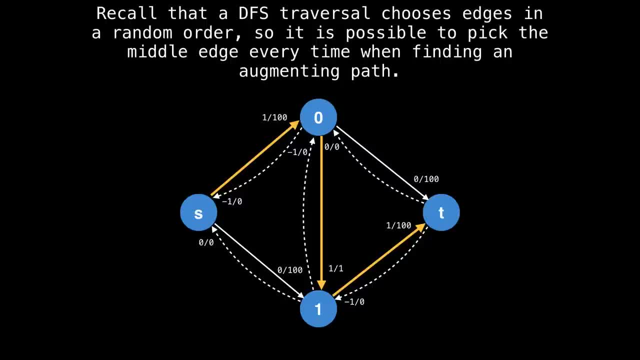 is essentially random. So it's possible for you to pick that middle edge with a capacity of one every single time, And what that will do is it'll limit flow. you can push from the source the sink to be one, So one is always going to be your bottleneck value, So you're. 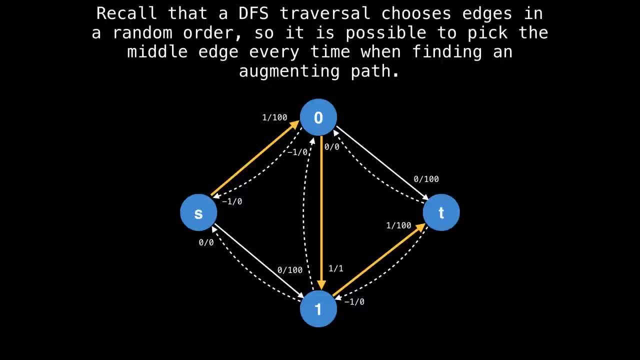 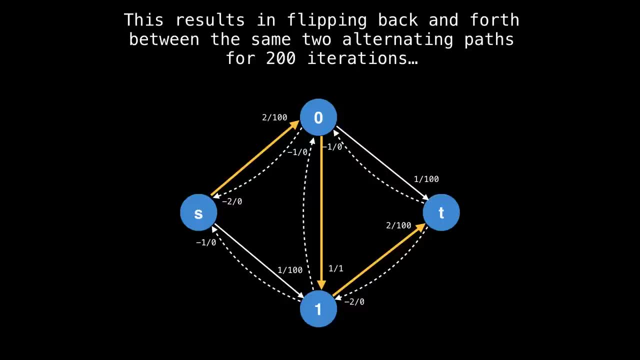 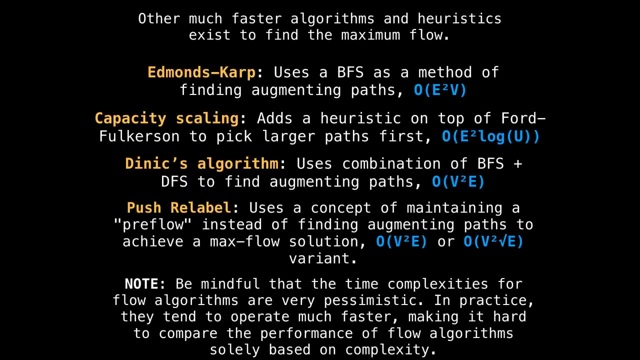 never going to be able to augment the flow by more than one unit. This results in flipping back and forth between the same two alternating paths for 200 iterations, which really kills your time- complexity. Luckily, much faster algorithms and better heuristics exist to find the maximum flow value. One example is: